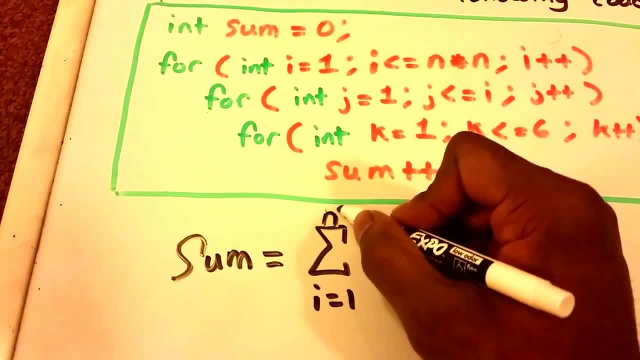 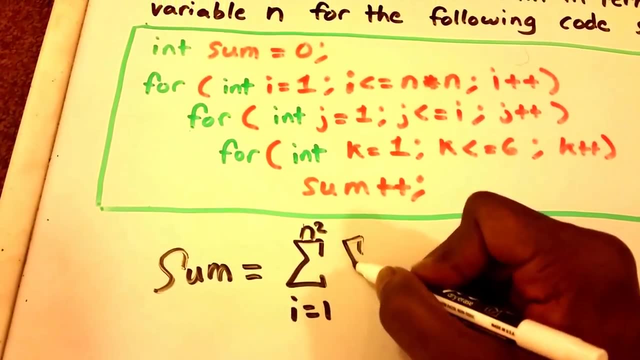 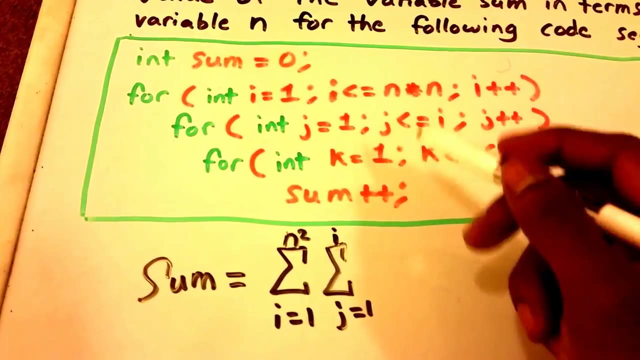 which is just n squared, And then, within that for loop, we have our second for loop. So we're going to have a second summation here, And the second summation is going to run from j equals one all the way to i, And then, within that second for loop, we have a third for loop. So we're going 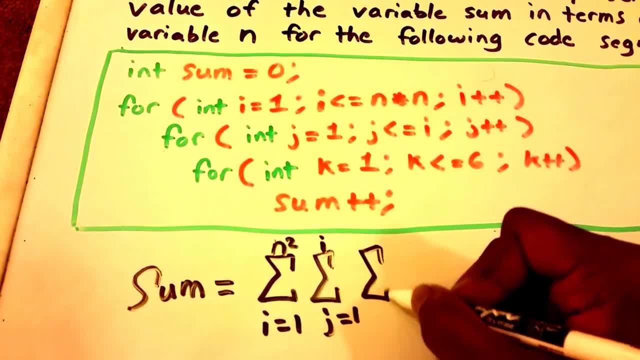 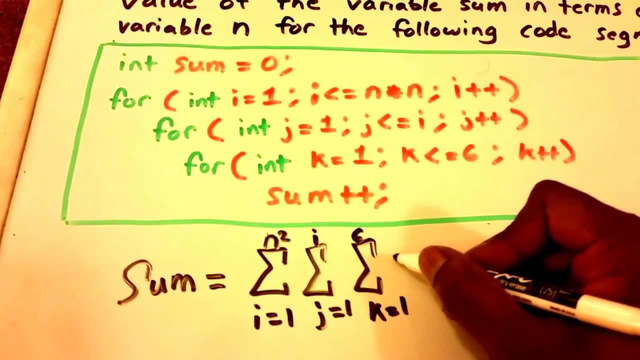 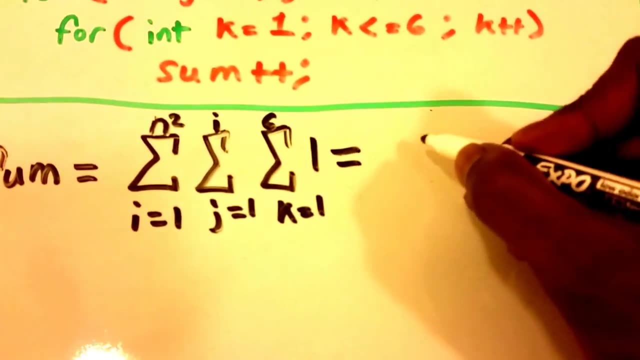 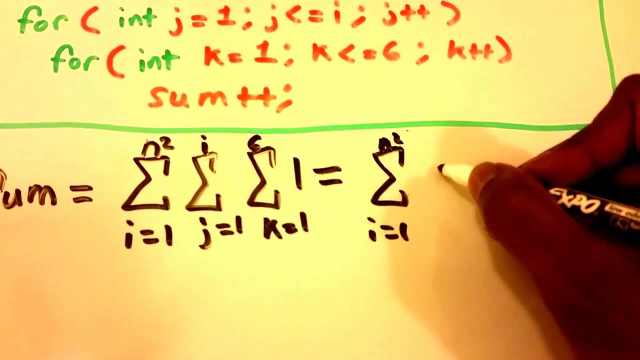 to have a second summation here, And that third summation is going to run from: k equals one to six of one. All right, So let's go ahead and simplify this. So now we're going to get the summation from: i equals one to n squared, And then within there we're going to get 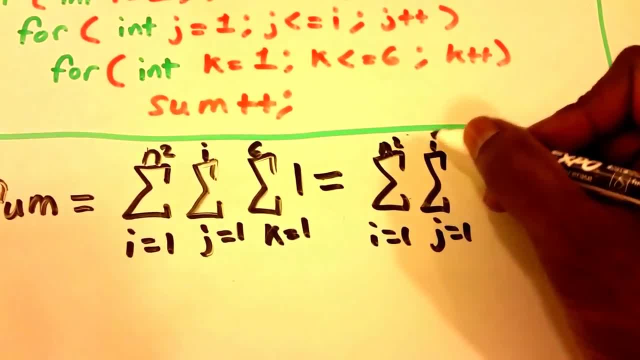 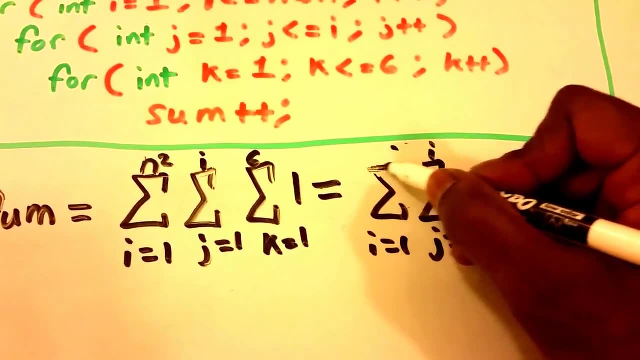 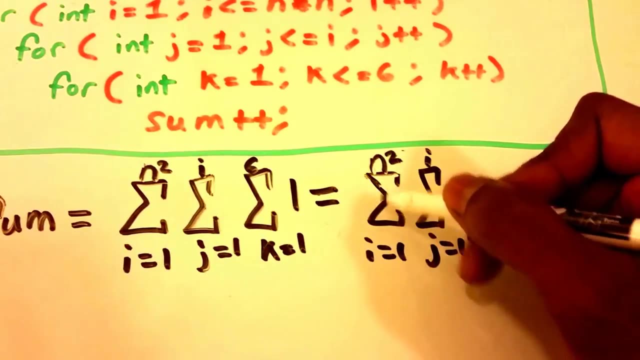 the summation from j equals one to i, And that's n squared. Let me make sure I write that a little bit better. Yeah, not much better, But you guys get the gist. That's n squared. Okay, this just becomes six. 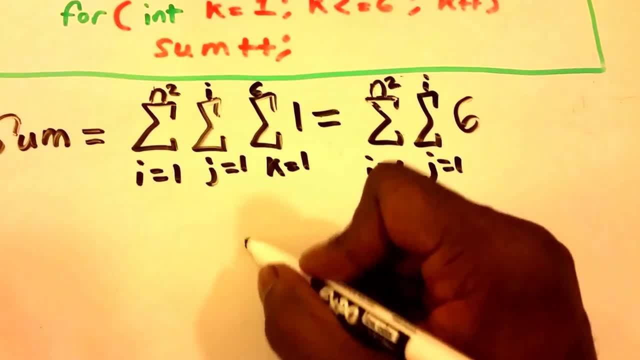 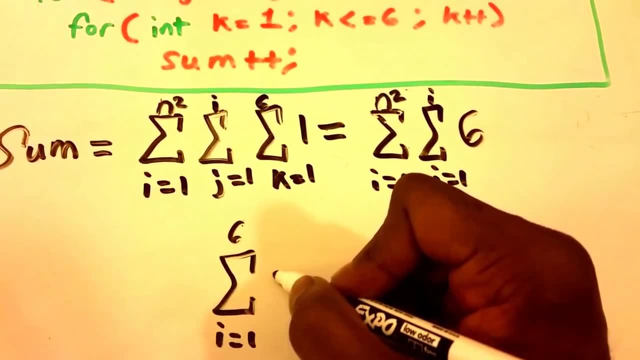 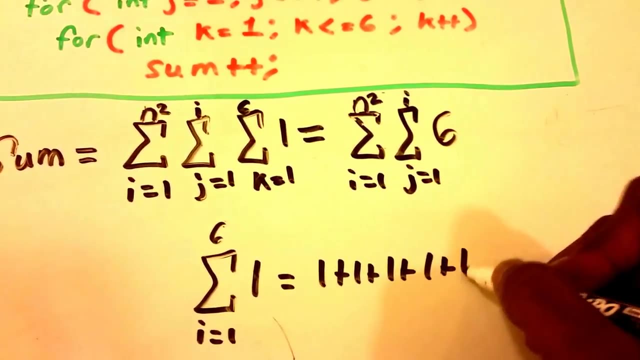 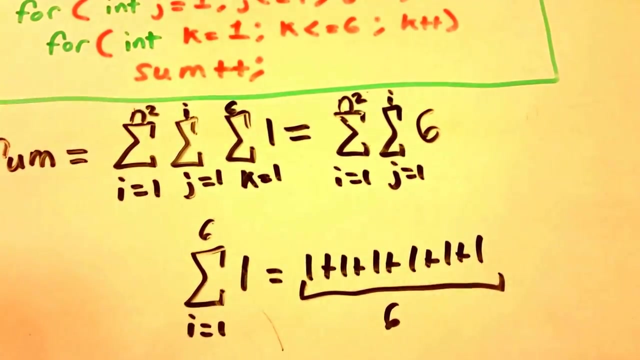 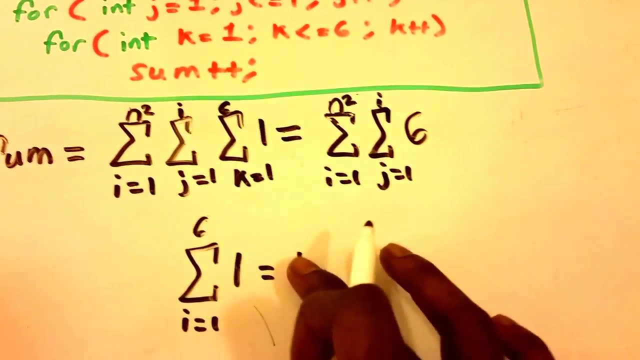 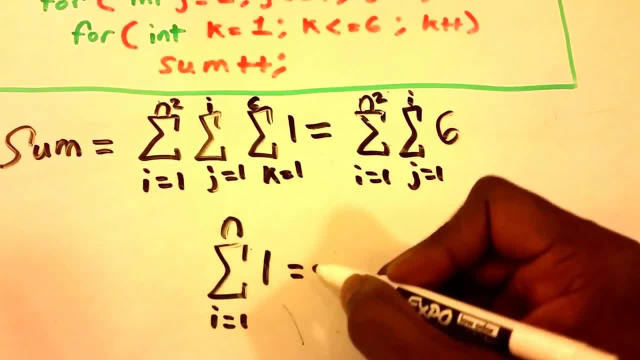 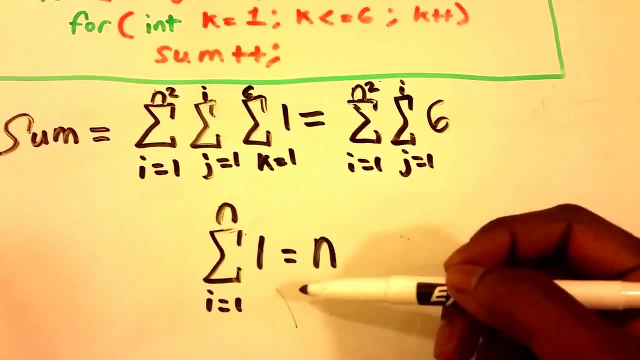 no matter what that value at the top is, let's say it's some arbitrary value- it's going to always get hearted, to get a little coasted. Okay, because one equal that arbitrary value in. so this is what that summation formula that we 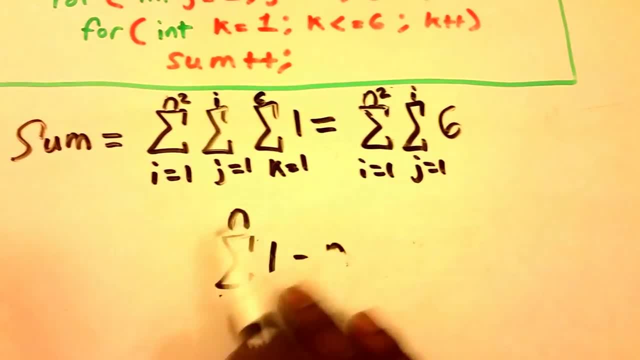 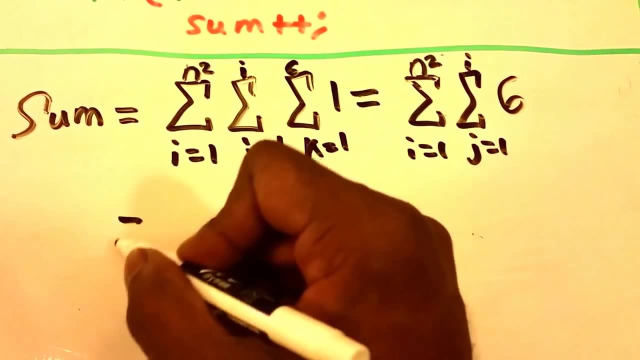 could use for our third summation here. alright, so I'm just going to erase this. so that's how I got the 6, and so let's simplify this a little bit more now. so now we're going to get the summation from: I equals 1 to n squared, and I'm 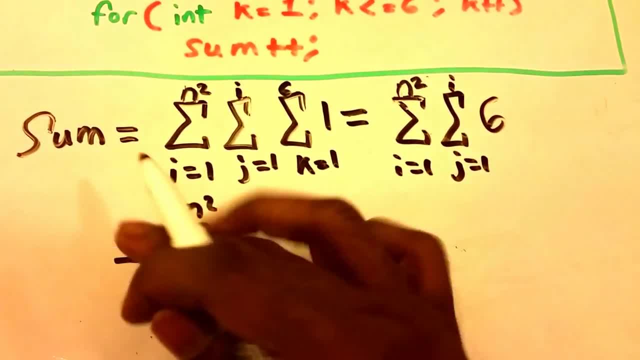 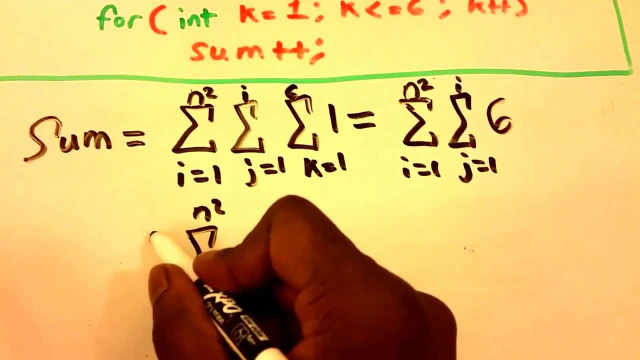 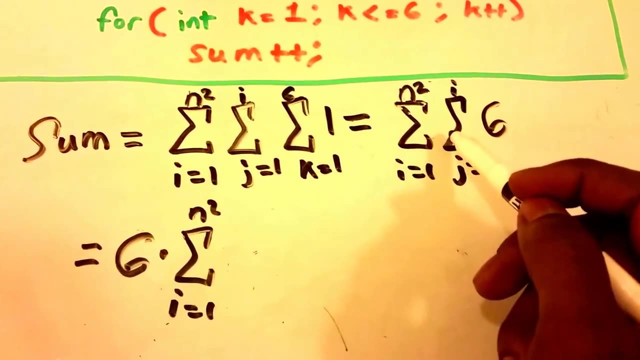 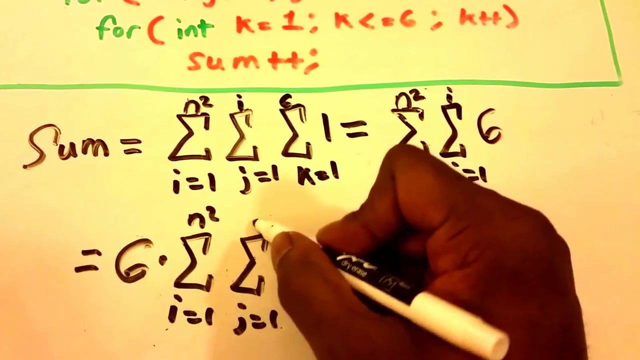 going to pull out that 6 here, so we have time 6, so time 6, and then we have that inner for loop right here, which is now the summation from J equals 1 of I of 1. so what does that equal? well, we're going to get the summation from I equals 1 to n squared, and I'm going to 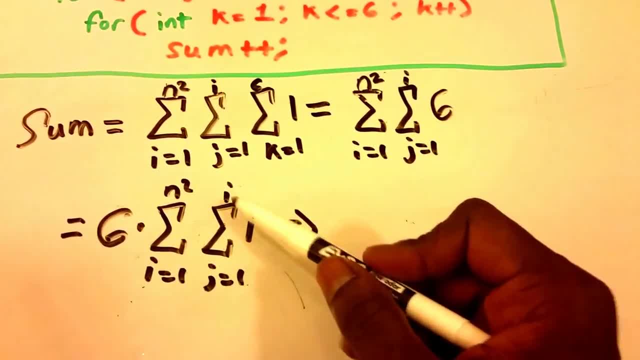 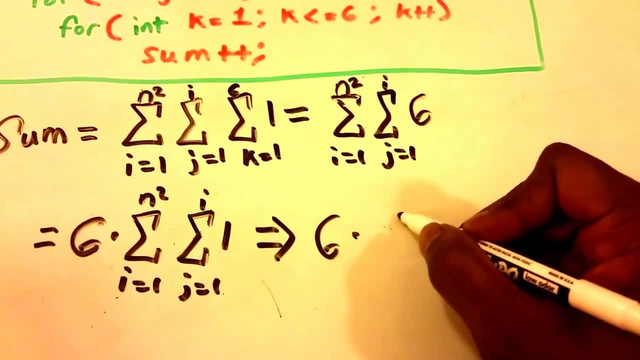 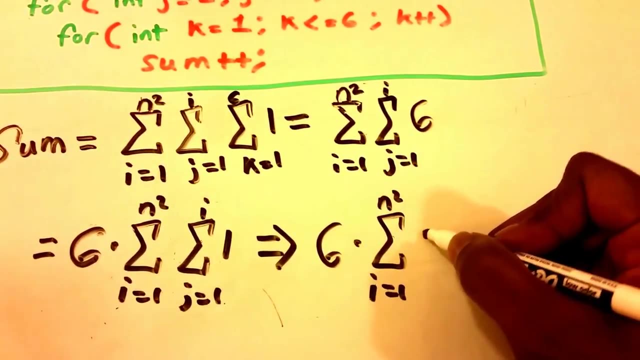 we just now. I just not showed you guys the formula. this is going to equal whatever that top variable is. so now we get 6 times the summation from: I equals 1 to n squared of I. so our second for loop just became I. alright, and then 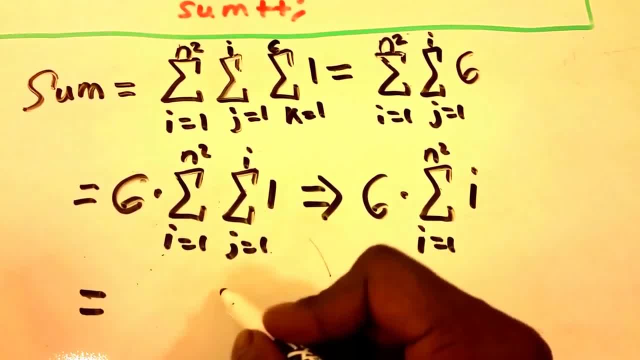 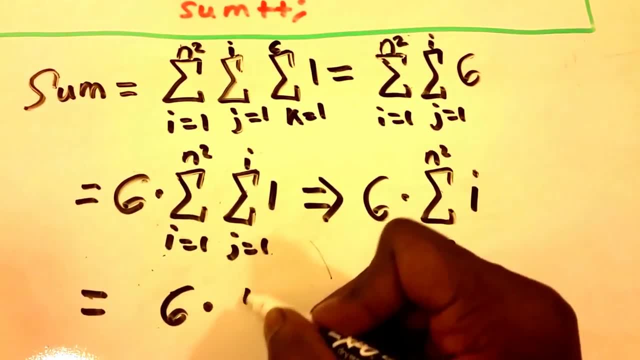 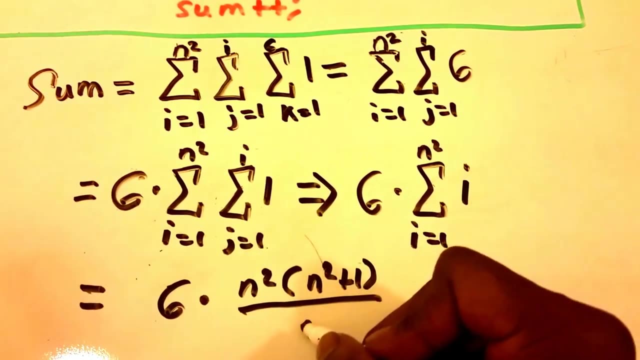 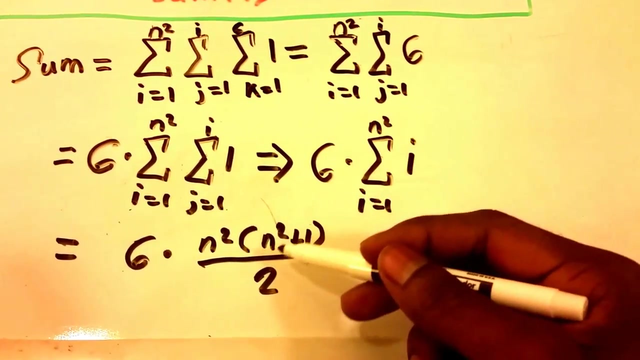 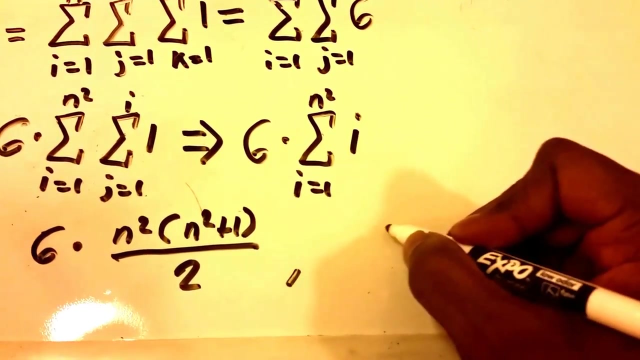 simplify this even more and we get 6 times n squared, times n squared plus 1 divided by 2. you may say, well, hold on here. how did you know that this summation here is equal to this formula here? and yeah, it's actually just another formula and I'm going to write it here. a. 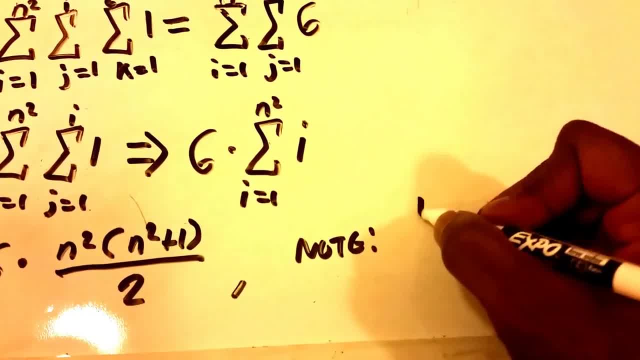 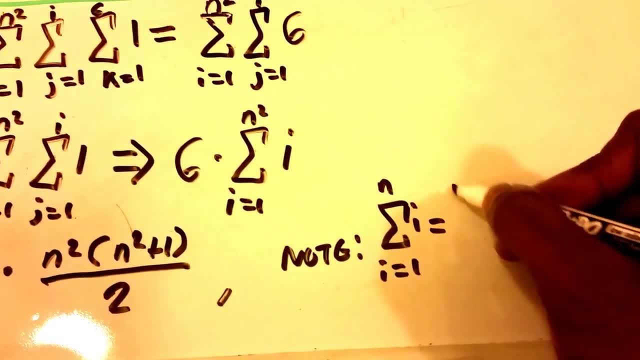 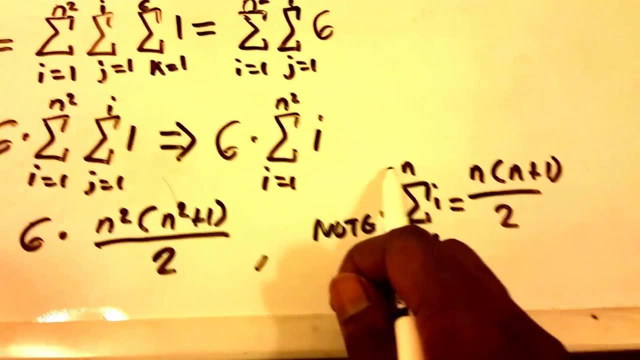 little note. The summation from i equals 1 to n, of i is equal to n times n plus 1 divided by 2.. So all I had to do was substitute that n up here for our n squared, and that's how I got this formula over here. 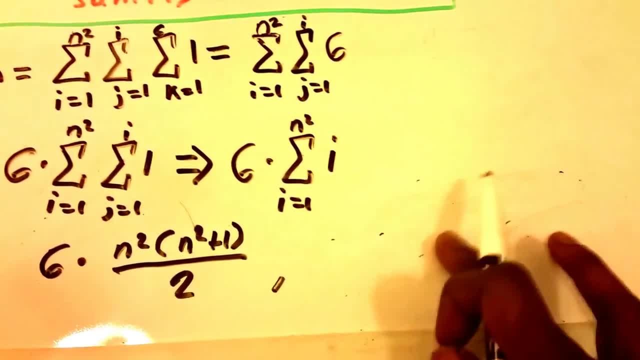 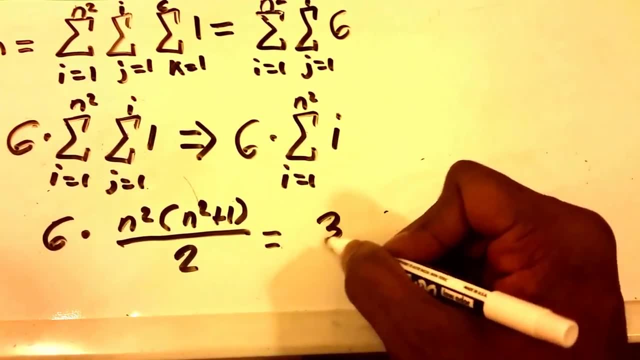 Okay, All right, so let's continue here. Okay, so now we're just going to get- I'm going to do a lot of simplifying here- actually 3,. well, no, I'll just write it all out. 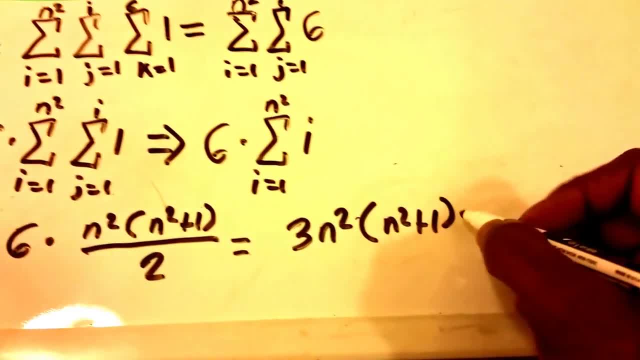 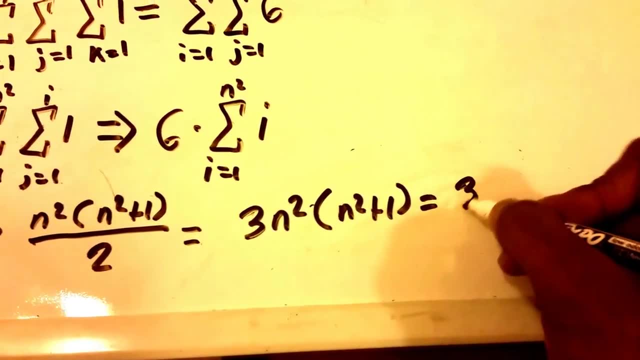 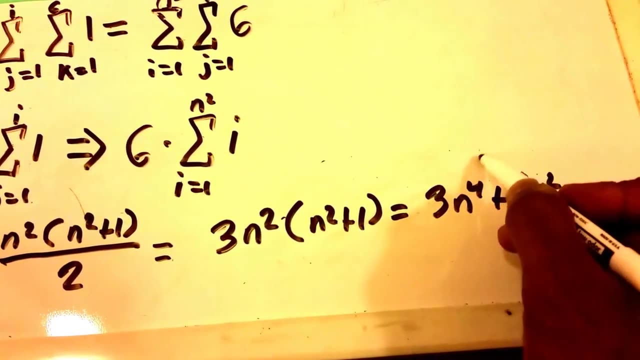 3 n squared, times n squared plus 1, because I just divided the 6 by 2. And then we're going to get 3 n to the 4th plus 3 n squared, And this is what sum will equal.